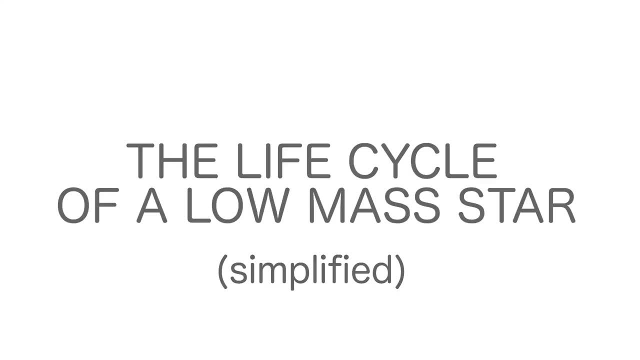 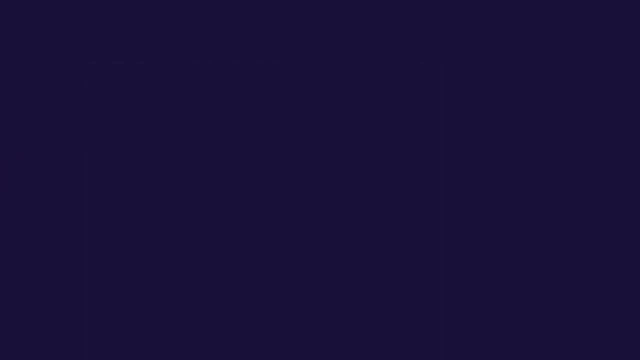 It's estimated that there are 300 billion stars in the Milky Way galaxy alone, which gets pretty terrifying when you consider that there are billions of galaxies in the universe. Each star has a different set of planets, rocks and even other stars orbiting it, and 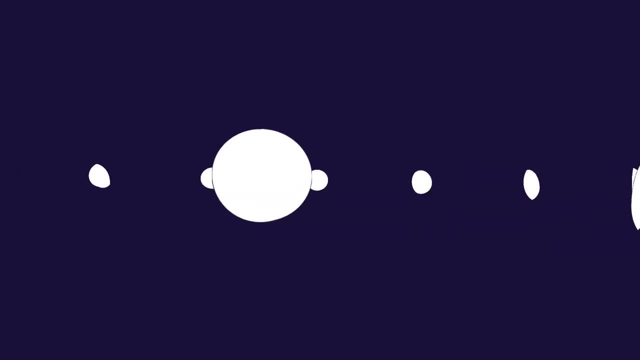 each star has a different life. However, we know the basic life cycle of a star and it's different depending on if it's a low-mass star or a high-mass star, but each one starts out the same: in a nebula. 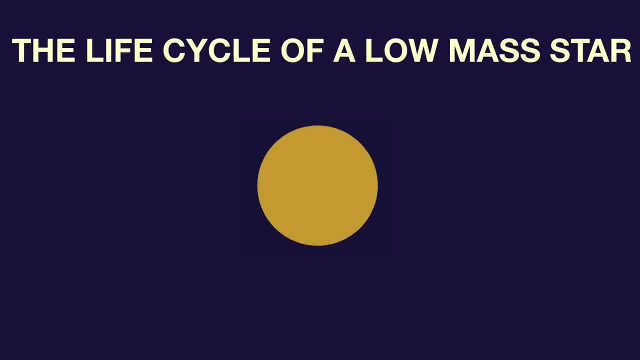 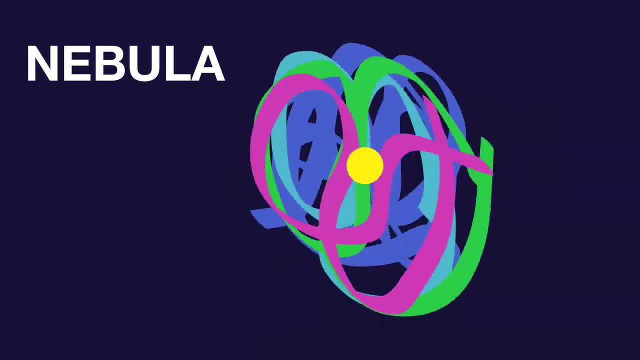 In this video we will cover the life cycle of a low-mass star. The star begins, just as we discussed in my last video. The nebula spins and spins and creates a center mass, but before the hydrogen starts burning, it's known as a protostar or a baby star. The 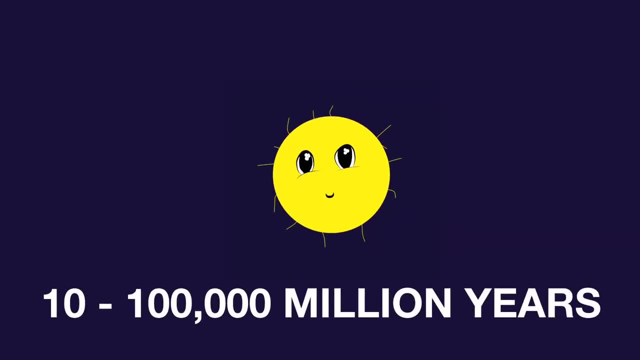 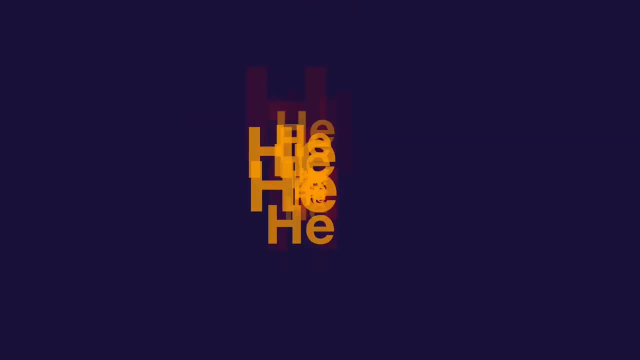 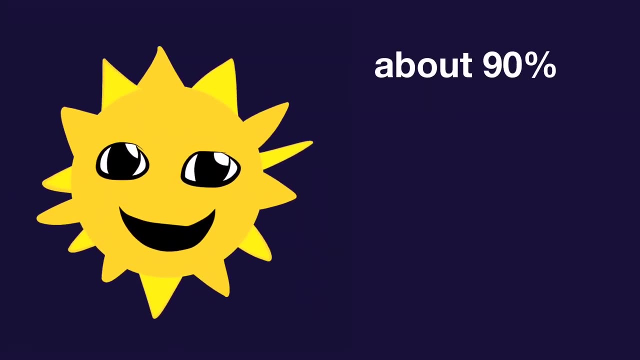 protostar will stay in this stage for anywhere between 10 and 100,000 million years, depending on the size of the star. Once the hydrogen begins to fuse helium, it becomes a main-sequence star. A star will live most of its life as a main-sequence star. In fact, about 90% of known stars are. 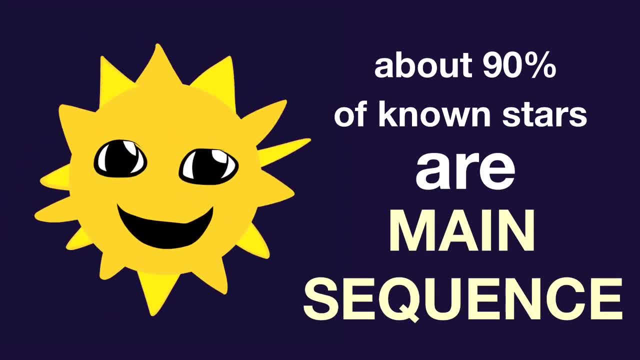 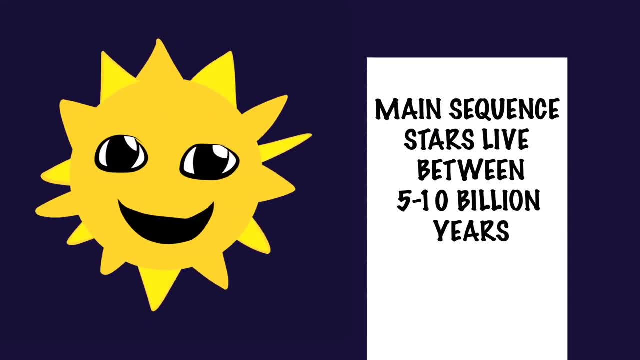 main-sequence. Our very own Sun is a main-sequence star and for our sake let's hope it stays that way for a long time, because in about 5 billion years a main-sequence star will begin to burn its helium, And when the main-sequence is all out of hydrogen to burn, it becomes 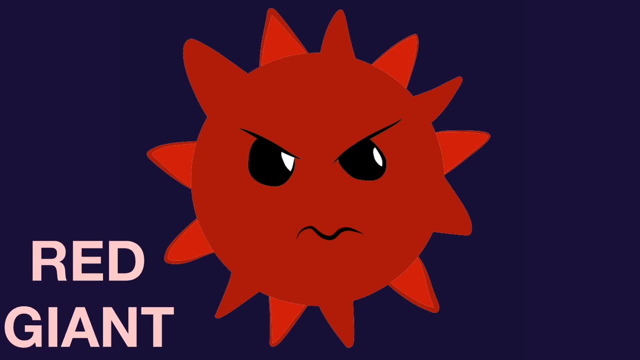 a red giant. A red giant is exactly what it sounds like: Red and giant. It burns red because its outside layer has a lower temperature, around 5000 Kelvin, whereas a main-sequence star could burn as hot as 40,000 Kelvin. As for the giant, our Sun will slowly get bigger and bigger. 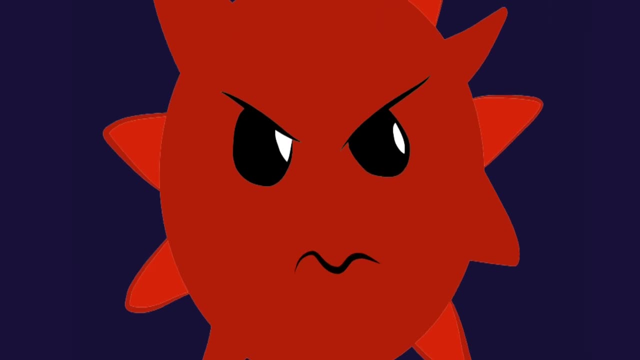 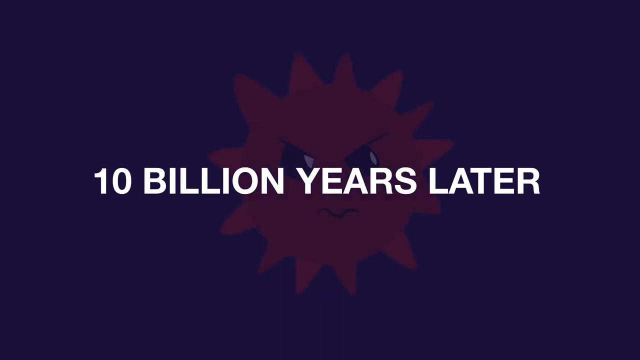 as it burns helium, it will absorb Mercury and Venus and scorch the surface of the Earth, making it uninhabitable. Yikes, After about 10 billion years, the red giant will become unstable. After 10 billion years, the red giant will become unstable and its core will no longer. 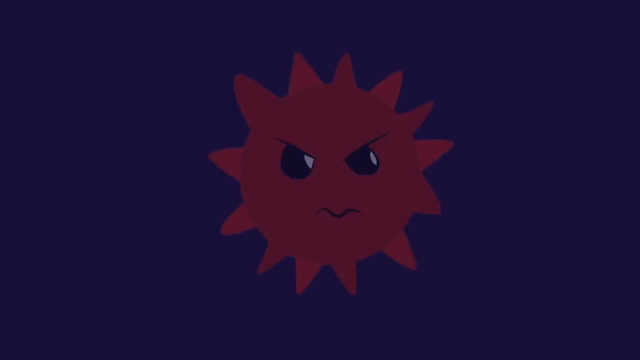 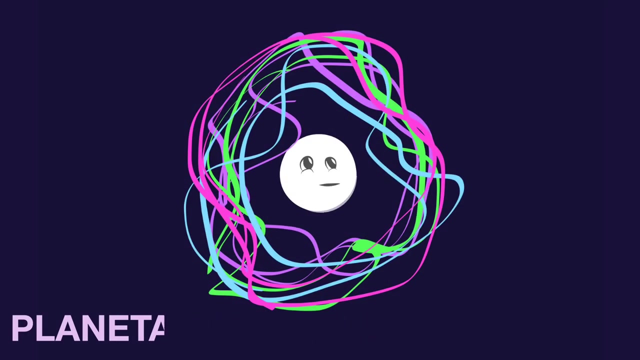 be able to hold the outer shells of the star. The outer shells will separate from the core of the star and create what is known as a planetary nebula. In the center there remains a white dwarf star. After a few thousand years, the planetary 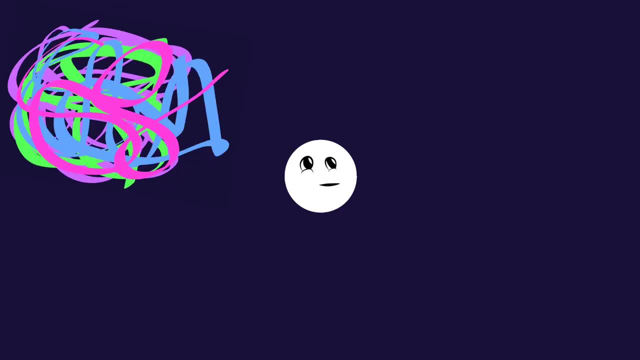 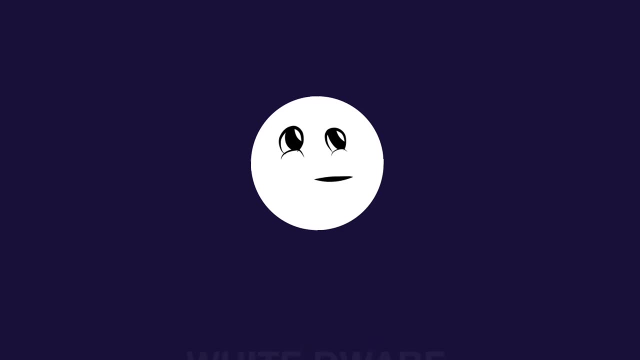 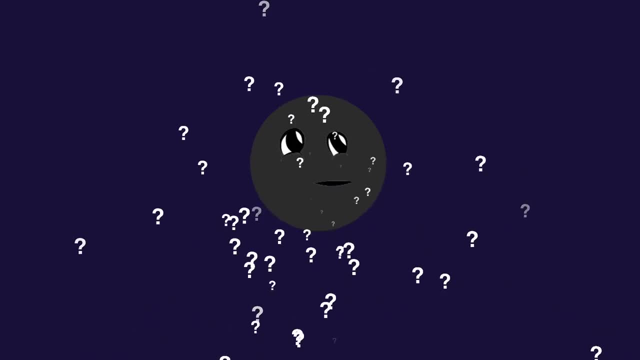 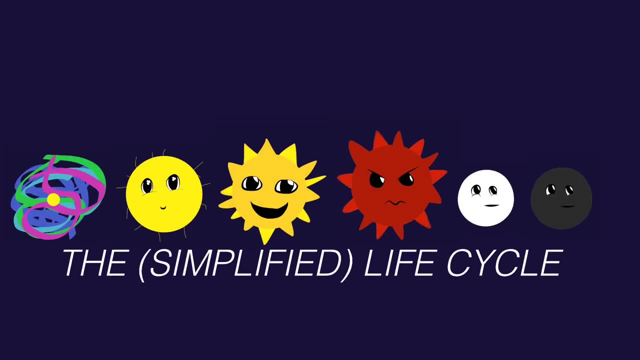 At least that's the theory. Scientists do not know 100% of the black dwarf star because we have never discovered one, but it is the most plausible guess given what we know, And that is the simplified life cycle of a low mass star. 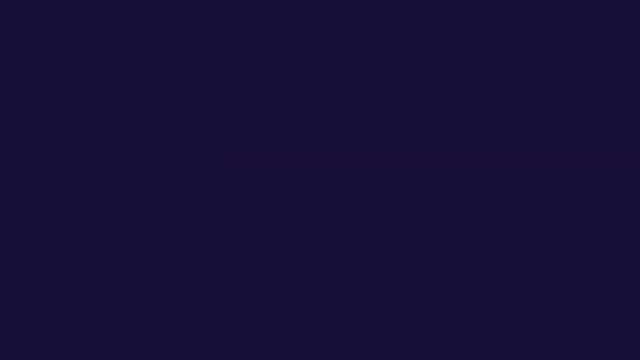 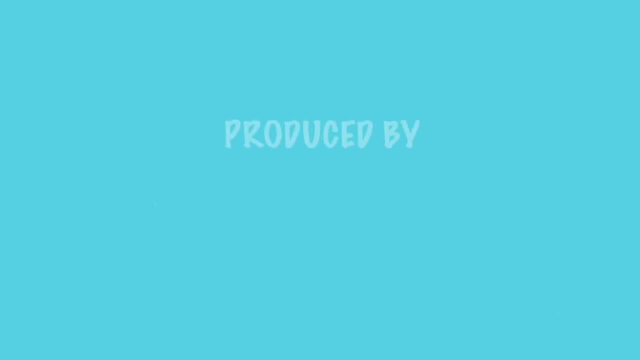 Thank you guys so much for watching. I really appreciate all of your support. Please drop a like and subscribe if you want to see more Earth and Space videos. See you next time, Bye, bye. 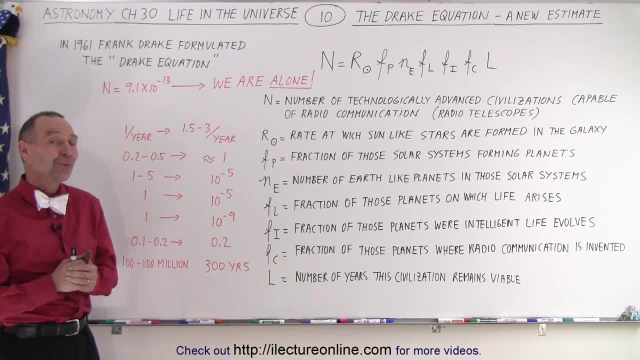 Welcome to Elector Online. So in the last video we saw how optimistic Frank Drake was, the one that came up with the Drake equation. He estimated that there might be as many as millions of planets in our galaxy that had intelligent life capable of communicating. 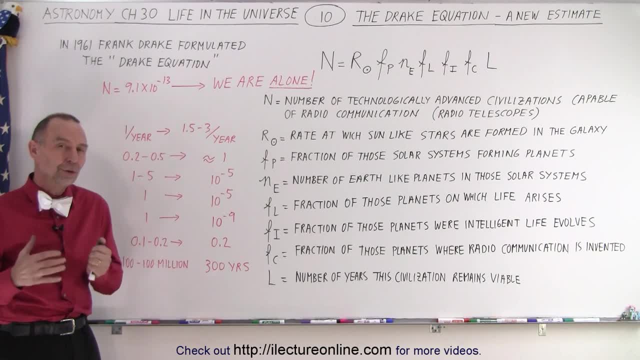 with us via radio communication. But since then we've learned a lot. That was back in 1961, and now we realize that the possibility of life arising on a planet, even if all the conditions are just perfect, are probably very, very remote, And so new estimates that we then place into the 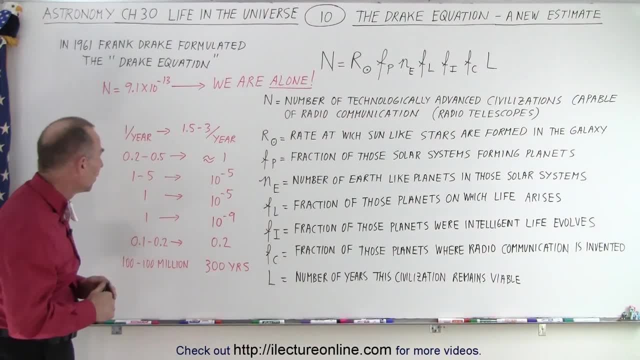 Drake equation gives us a very different result. Let's take a look. First of all, the number of solar light stars that would form every year. we went from one per year to a more optimistic 1.5 to 3 per year. In a thousand you're 100 again. Oh, all right. So we estimate that. now we